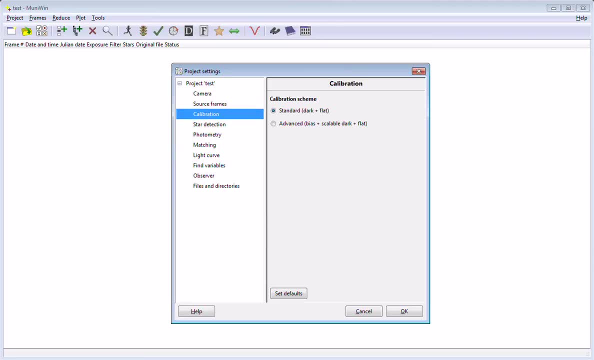 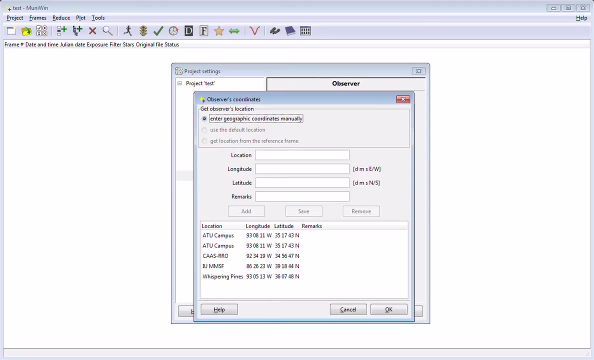 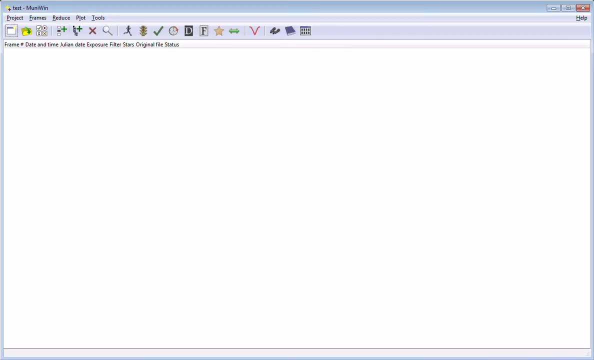 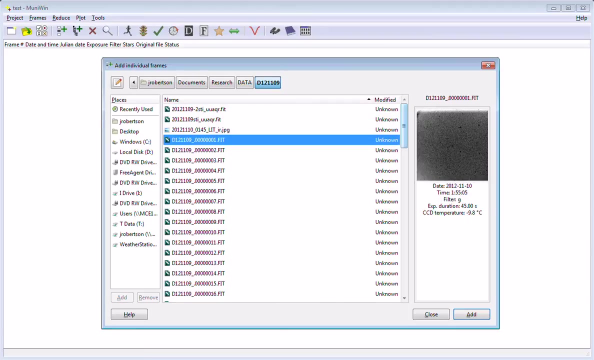 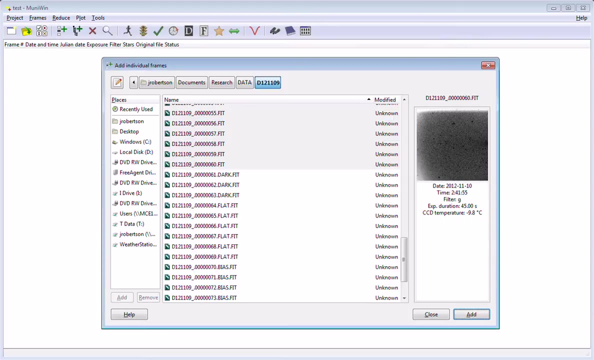 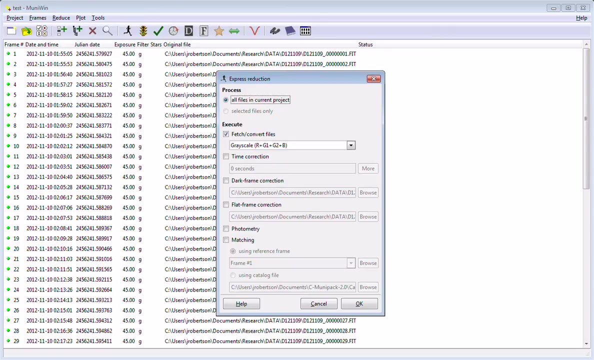 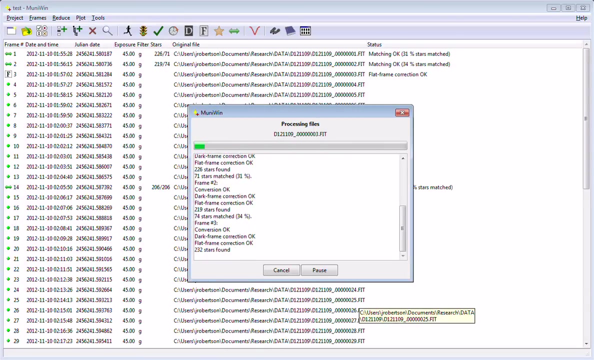 Make sure everything looks like there's nothing strange going on. Pick an observatory Where the data was taken, Find the files that you want to use, Choose your calibration And do the photometry. Once the photometry is finished, all the stars will be pattern matched and lined up and they'll extract. 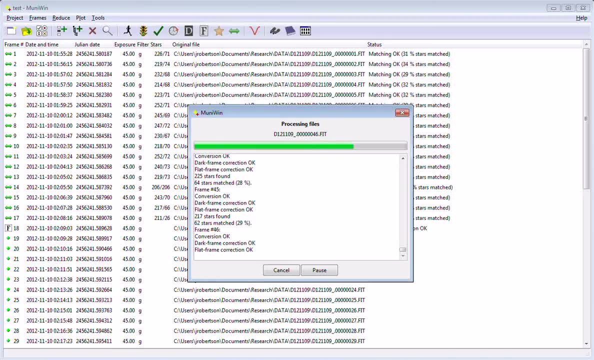 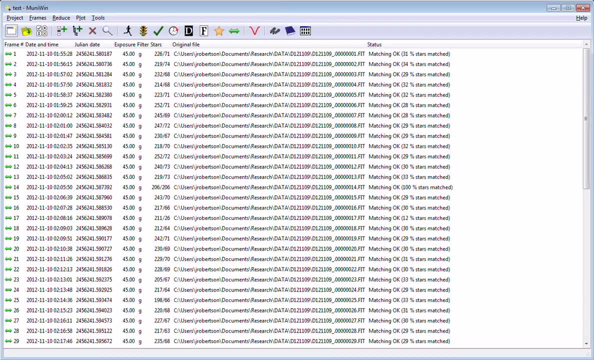 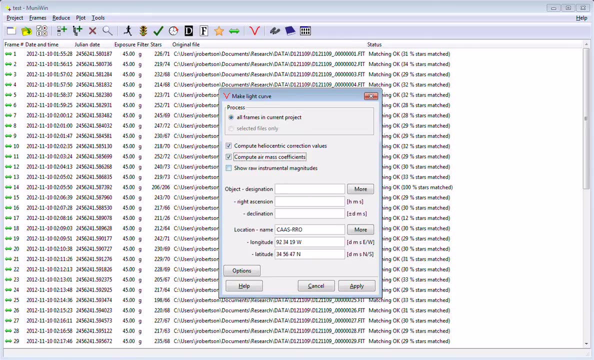 the magnitude of your variable and comparison stars that you choose on the default image. If you've chosen the observatory correctly, now when you choose the coordinates for the star, it will allow the heliocentric correction to be applied in the right manner. 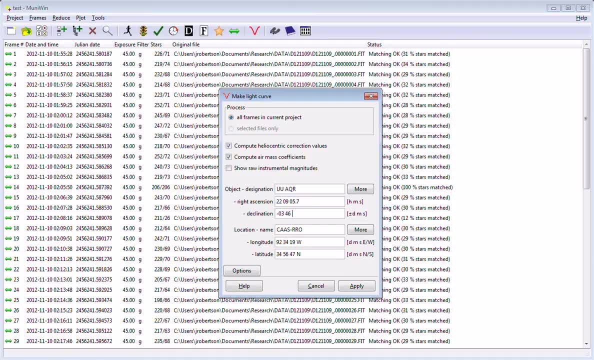 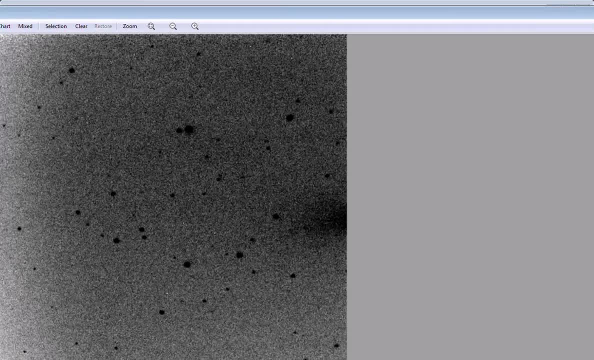 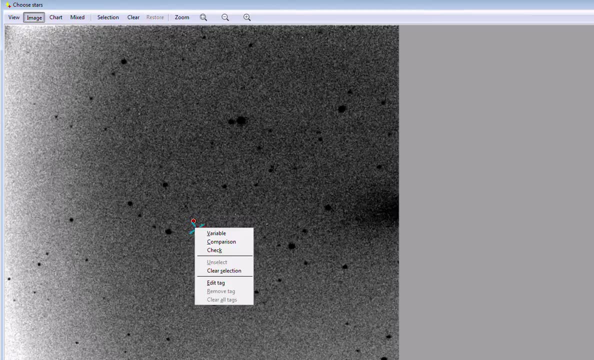 so that you'll have heliocentric Julian Day as output, if you chose that, And now all we have to do is choose the stars that we want to be extracted. You can have multiple comparison and check stars. That just means you'll have extra columns in your data. 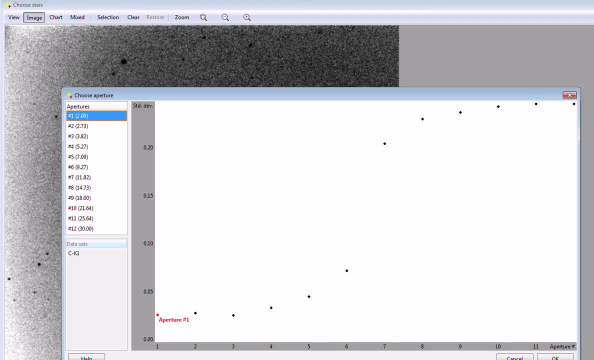 Three is enough. Sometimes one of these other apertures will be less noisy, Sometimes the third or fourth aperture, but it definitely goes up as the aperture goes up and includes more noise and sky and other stars. So usually the first aperture is the best.